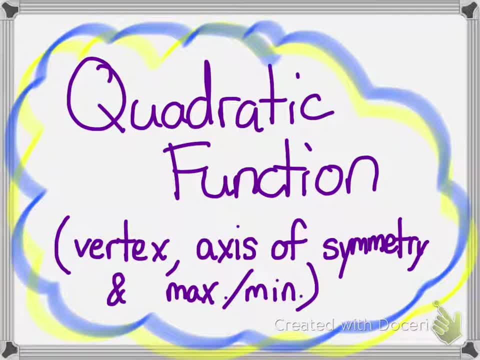 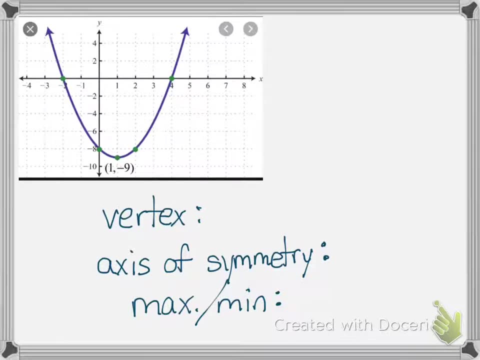 Hello everybody. Alright, in this video I'm going to show you guys how to find the vertex, axis of symmetry and the maximum and minimum of a quadratic function from the graph. Alright, let's look at our first example Now. your vertex is always going to be the highest point or the lowest point of your parabola. 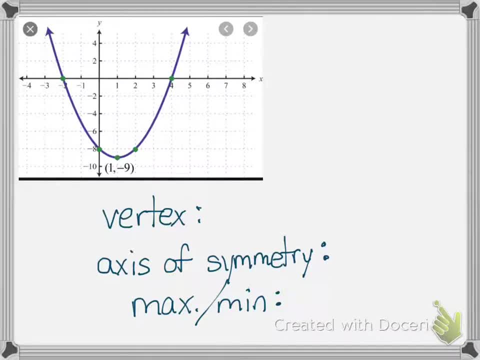 And when you identify where that point is, you write the order pair. that's your vertex. So, looking at this first example, my lowest point is right here And the order pair of that point is 1, negative 9.. So that's my vertex. 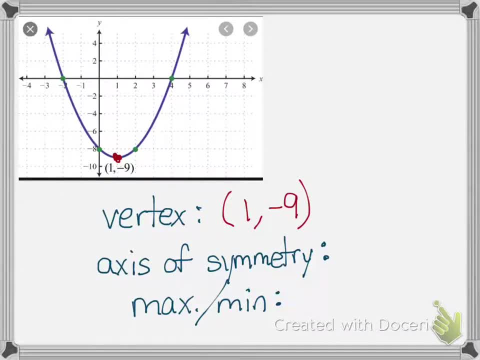 My axis of symmetry is always the imaginary line that goes straight through your vertex. So here's my vertex. If I'm going to draw a vertical line that goes straight through it, it's going to look just like that. Now you have to determine where on the x-axis did that dotted line just cross through? 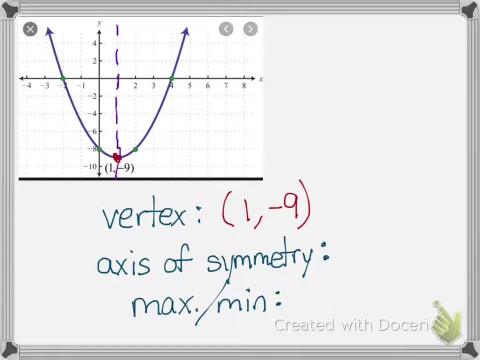 As you can see, it crossed through the number. So therefore, my axis of symmetry is x equals 1.. And since my vertex was the lowest point, I have a minimum. Alright, let's look at another example. Again, your vertex is the highest or the lowest point of your parabola. 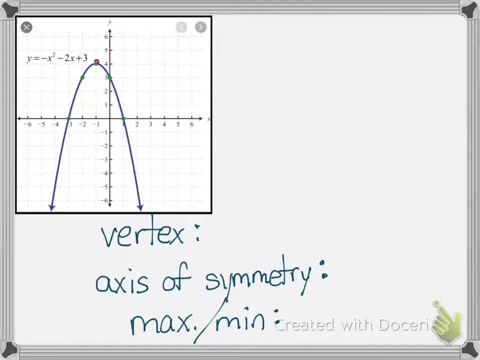 As you can see in this parabola, my highest point is up here. I don't have a low point because I have arrows down there. So the order pair of that point is negative. 1, comma 4.. Remember, axis of symmetry is the dotted line. 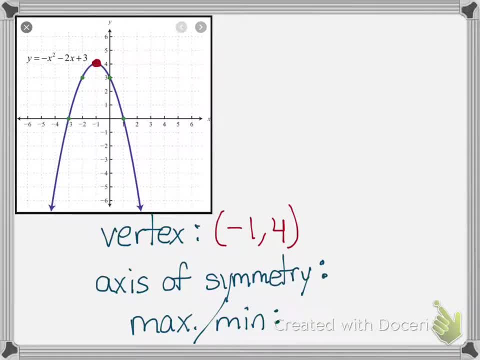 That goes straight through your vertex. So if I was to draw a dotted line that goes straight through my vertex, it will look just like that And it will cross over the x-axis at the number negative 1.. So therefore, my axis of symmetry is: x equals negative 1.. 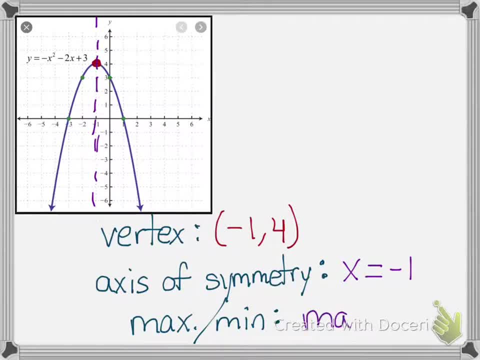 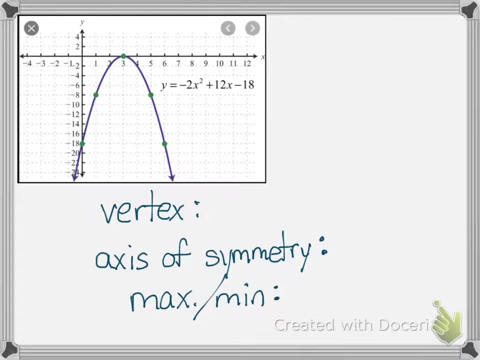 And, of course, since my vertex was up top, I do have a maximum point. Alright, let's look at the next example. Remember, vertex is the highest or the lowest point of your parabola. In this particular example, I have a point up here. 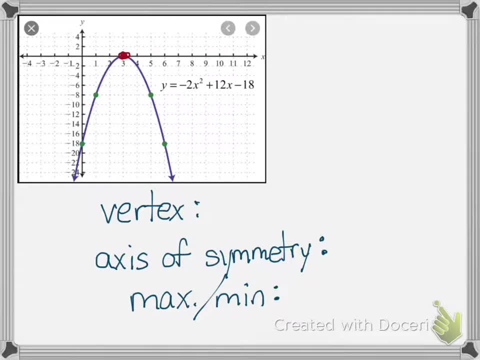 I have a point up here on top of my parabola, So my vertex is going to be 3, comma 0. And again, your axis of symmetry is the imaginary dotted line that goes straight through your vertex. As you can see, my dotted line crosses the x-axis at the number 3.. 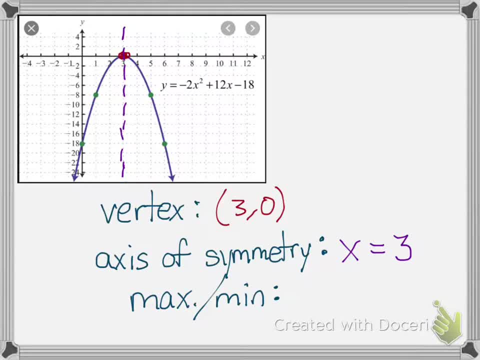 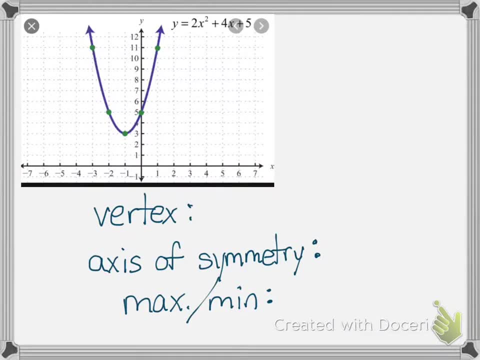 So my axis of symmetry is x equals 3.. And since that vertex is on top, I have a maximum. Look at this last example. My vertex, remember, is the highest or the lowest point of your parabola. So since I have a point down here, that's going to be my vertex. 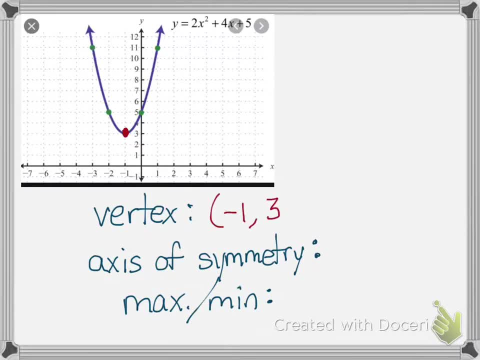 And the order pair of that is negative 1, comma 3.. My axis of symmetry is an imaginary line that goes straight through your vertex And, as you can see, that dotted line crosses on the x-axis at the point negative 1.. 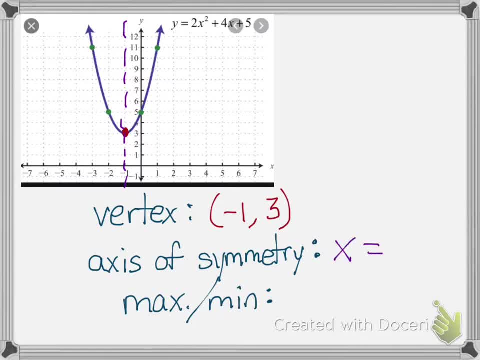 So my axis of symmetry equals x, equals negative 1. And again, since my vertex is at the bottom, I have a minimum And that's it.